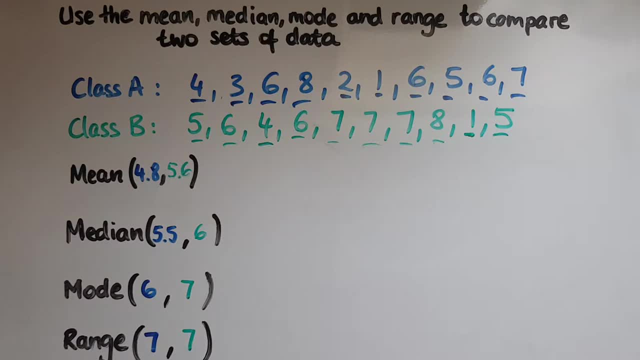 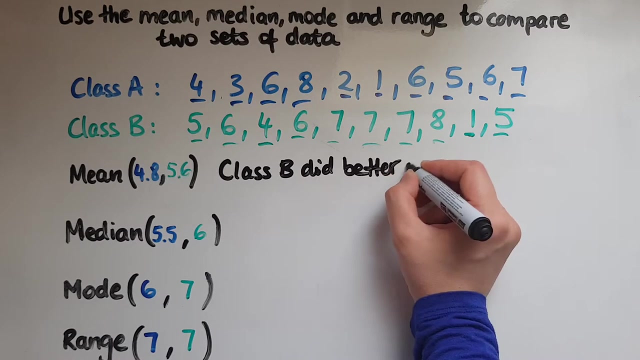 So what does that tell us? Since this is an average measure, the mean that tells us that class B did better in general. Class B did better on average- That's a better word to use- And the median as well does about the average as well. 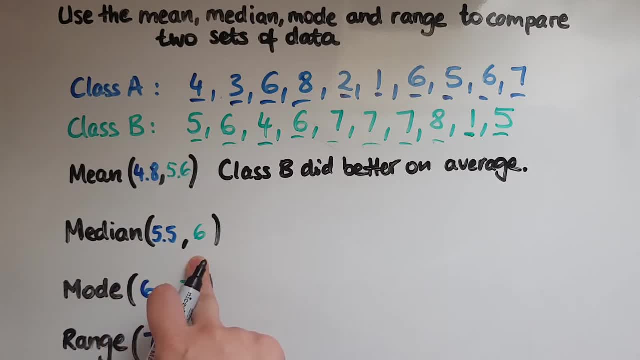 So that is supporting the same thing: That class B did better on average, because they received on average 6 marks, Whereas class A 5.5 marks. So Again, this supports the same thing: That class B did better on average. 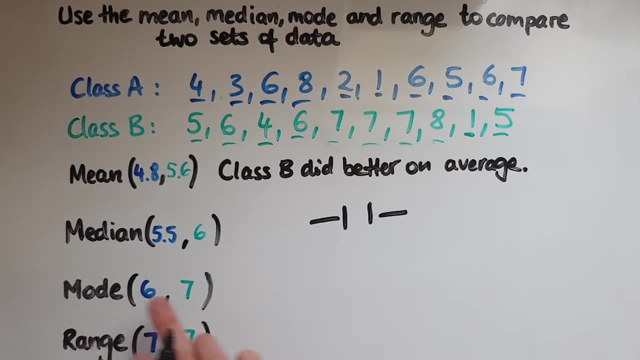 In terms of the mode, which is the most common value, the most common mark. This shows again that the most common mark for class B was 7. Which was one mark higher than for class A. So In terms of the mode, we can say that the most common mark was higher in class B. 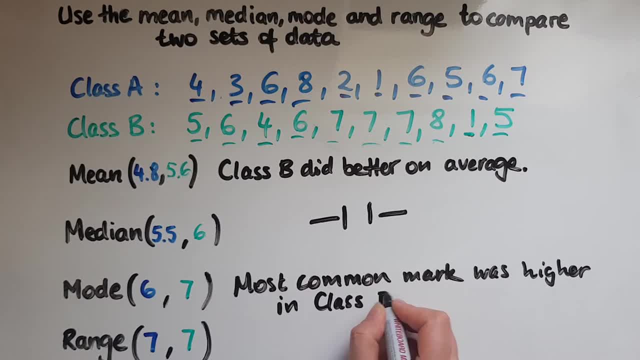 So That again supports the argument that class B did better. And in terms of the range, which we know is the difference between the highest and the lowest mark, That kind of measures, the spread, How spread out are these marks? And, As you can see from class A, the lowest mark was 1 and the highest was 8..